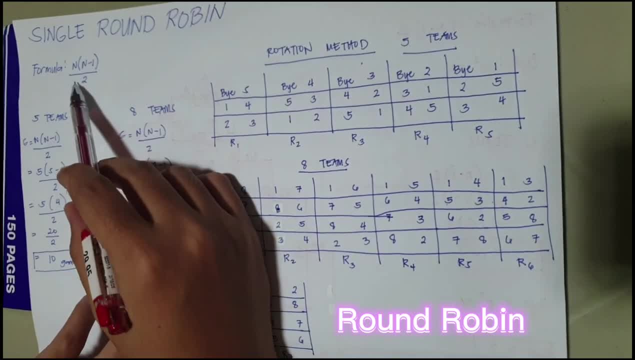 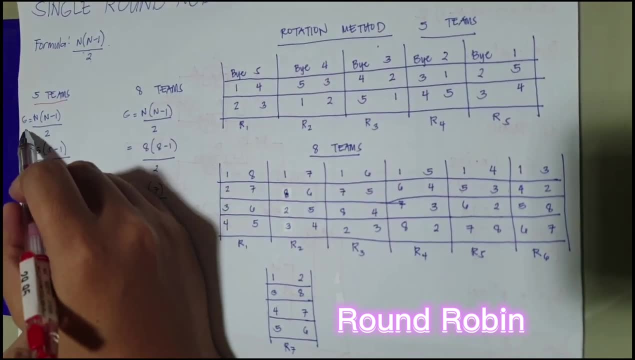 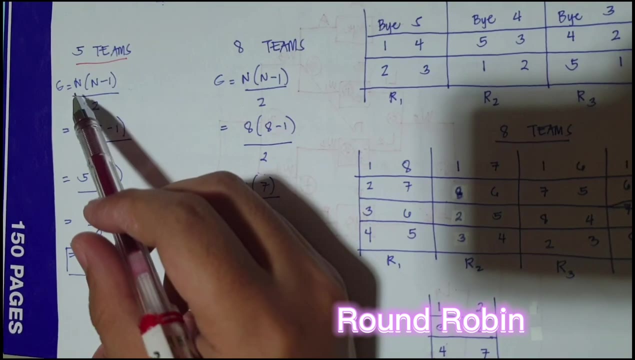 For the formula we're going to use: n times n-1 over 2.. So let's say, for example, 5 teams, So g equals n times n-1 over 2.. So we're going to replace n with 5, since n stands for the number of entries. 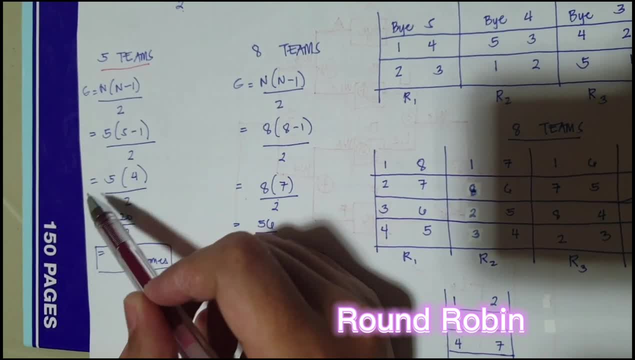 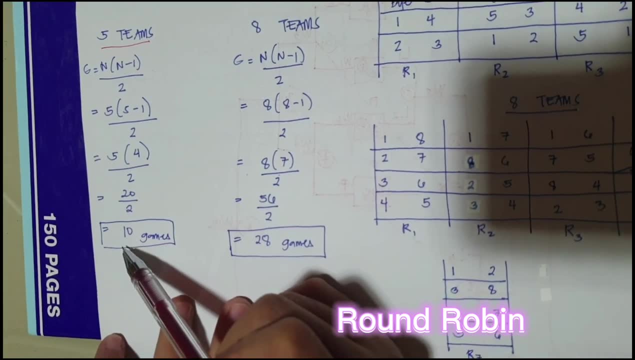 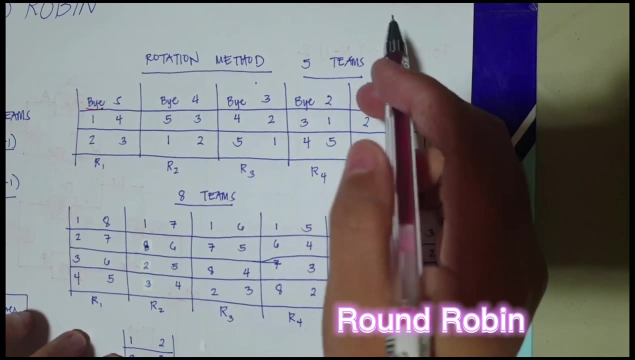 So 5 times 5-1 over 2.. So 5 times 4 over 2.. So 20.. Over 2 is equals to 10 games, So in rotation method for 5 teams. so by is applicable if the number of entries or the number of teams is odd. 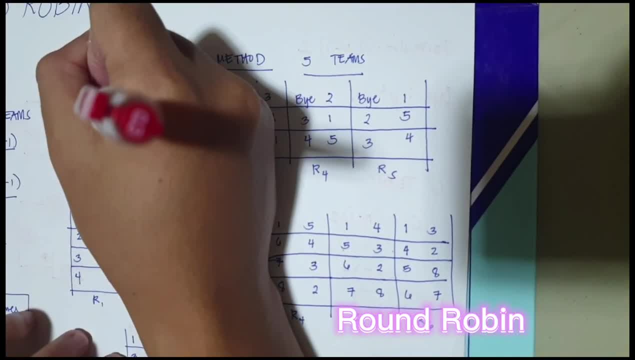 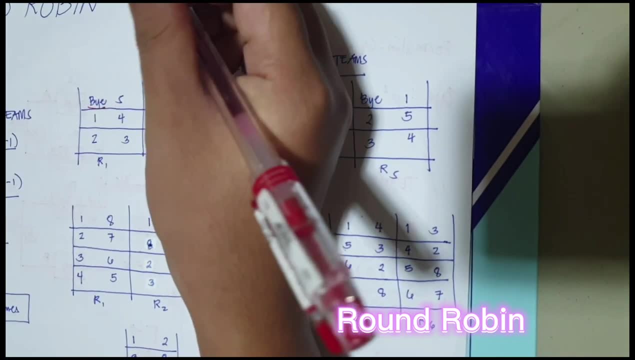 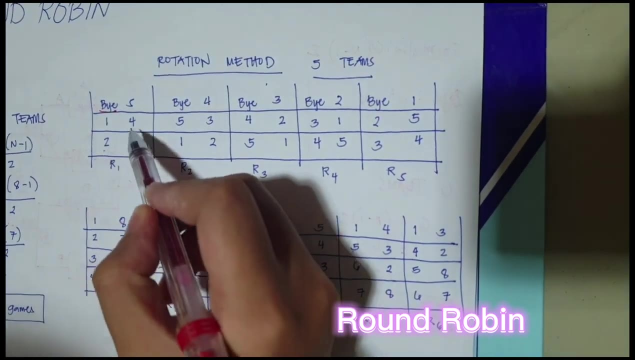 So by here is fixed, will remain fixed, and then the other numbers rotate around it in a counterclockwise direction. So let's say, for example: this is by: So there are 5 teams, So 1,, 2,, 3,, 4,, 5.. 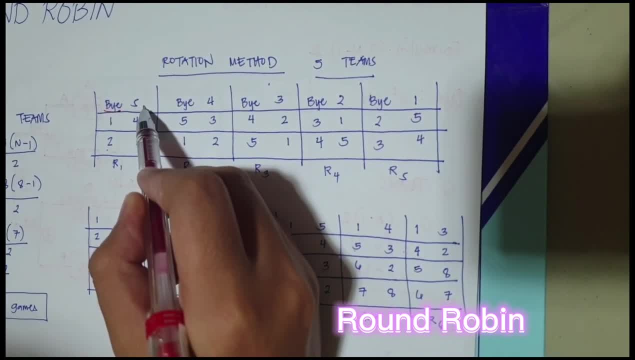 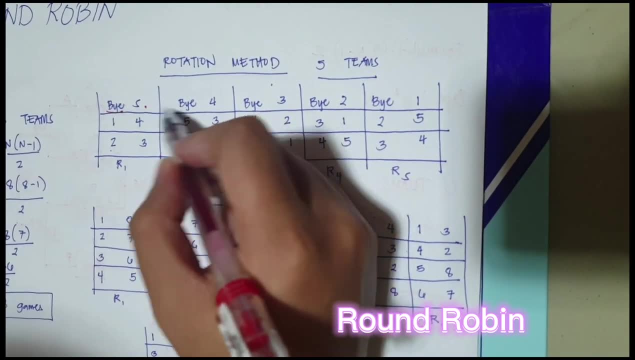 So we're going to rotate the numbers in a counterclockwise direction, meaning to say to the left. Okay, To the left, So for the next round, so by. So 5 is the number of entries, so it's fixed in the lower number by. 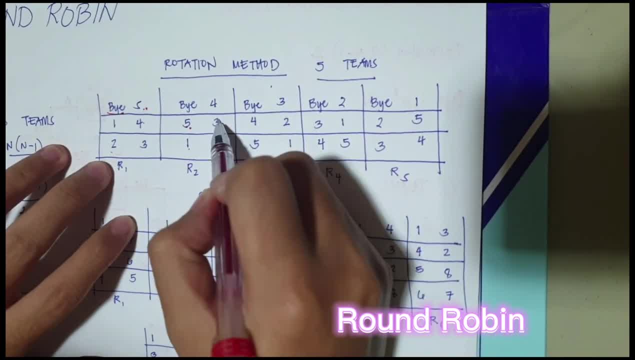 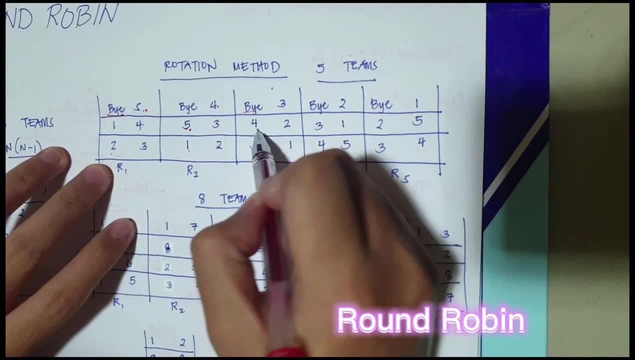 So 5,, and then to be followed by 1,, 2,, 3,, 4.. Then for the next round by: So next number is 3.. So 4 is fixed: 4,, 5,, 1,, 2,, 3.. 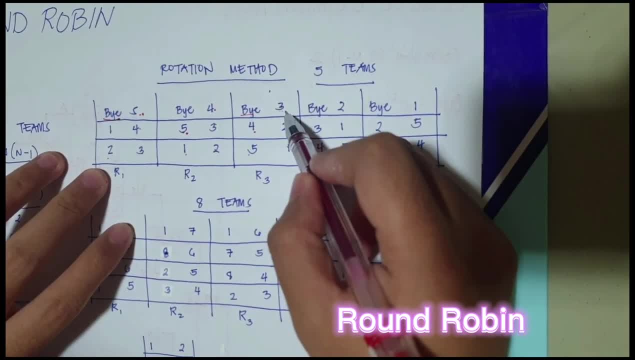 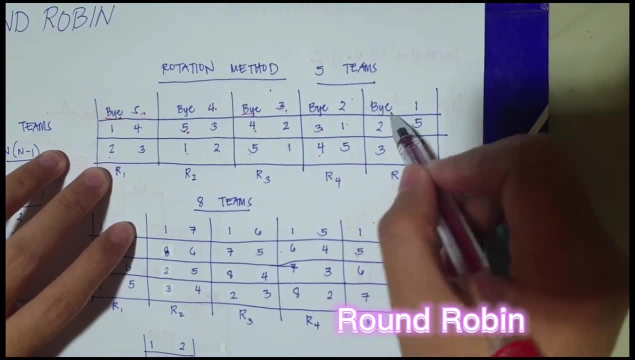 For the next round, by So 3 for the round 3.. So 3, 3,, 4,, 5,, 1,, 2.. And then, for the last round, 5, 2, by 2,, 3,, 4,, 5,, 1.. 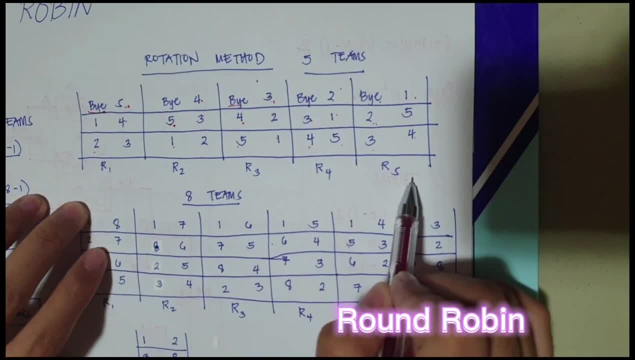 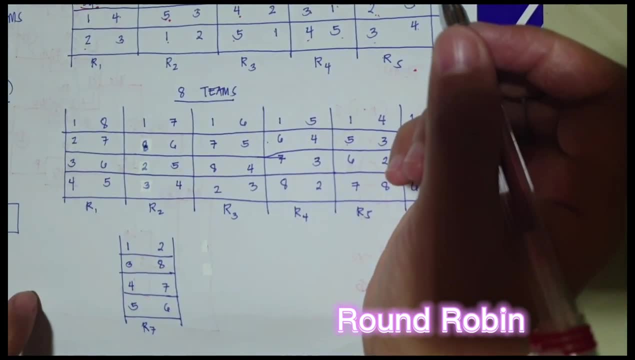 So all in all there are 5 rounds in 5 teams, So we're going to assign game number na. So there are 10 games. So, for example, this is the game number, So we're going to put 1 here. 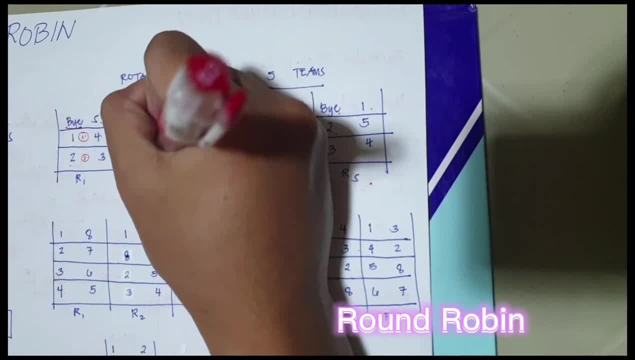 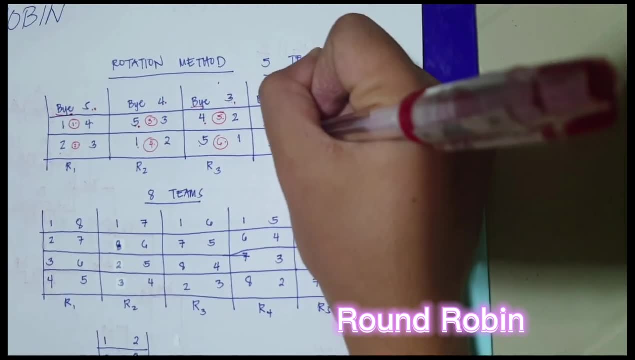 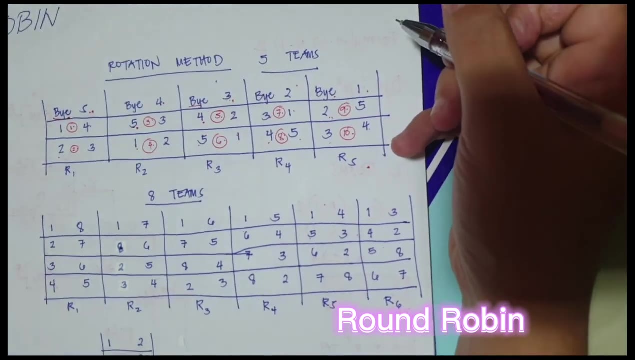 Game number: 2. Game number, 3. Game number, 4. Game number, 5. Game number, 6. Game number, 7. Game number, 8. Game number 9. Game number: 10. For the even numbers. so let's say for example, 8 teams. 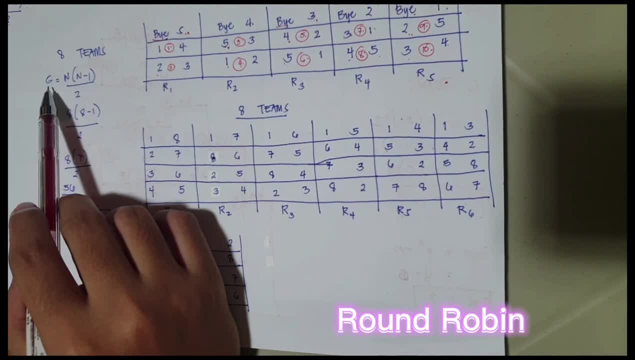 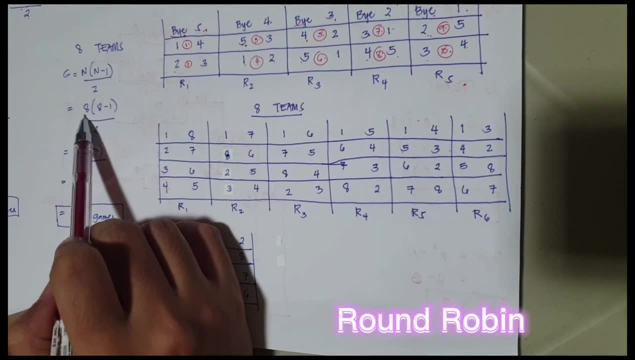 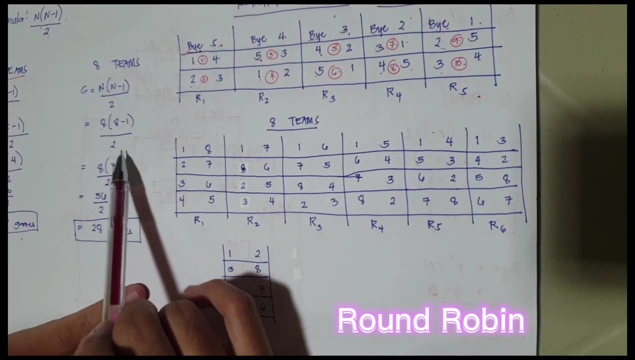 So we're going to compute the number of games Using the formula. So g equals n times n minus 1 over 2.. So we're going to replace n with 8.. Since there are 8 teams, So 8 times 8 minus 1 over 2.. 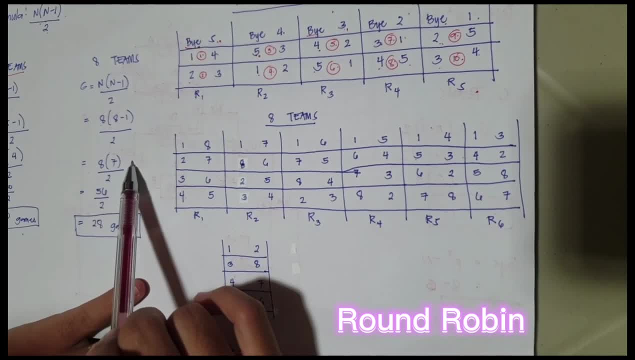 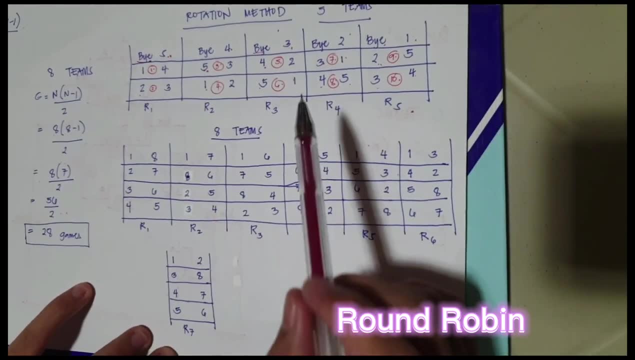 So 8 minus 1 equals to 7.. So 8 times 7 equals to 56 over 2.. So 56 over 2 equals to 28 games. So same with the rotation method in 5 teams, But then 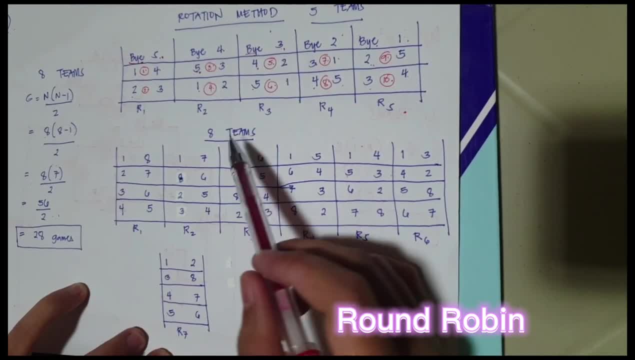 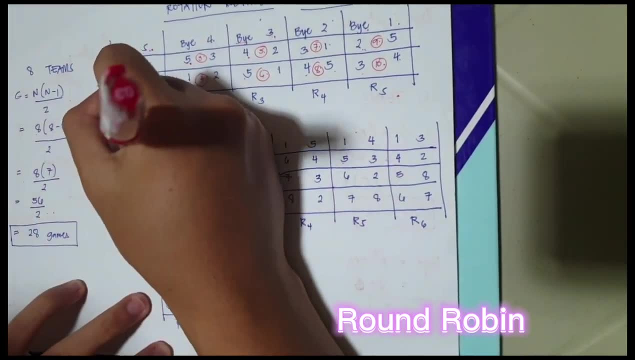 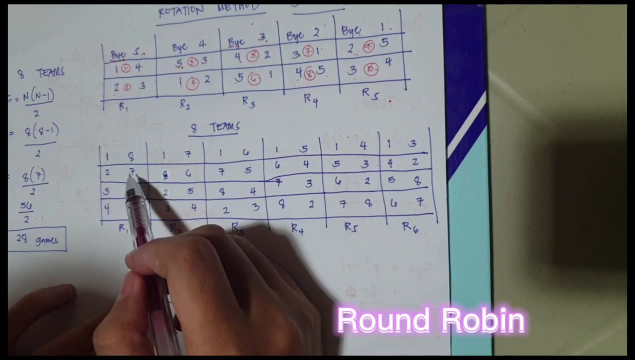 Since this is an even number, So the by here is not required, Okay Or not applicable. So let's say, for example, the 1 here remains fixed, And then the other numbers will rotate around it, And then in a counterclockwise direction. 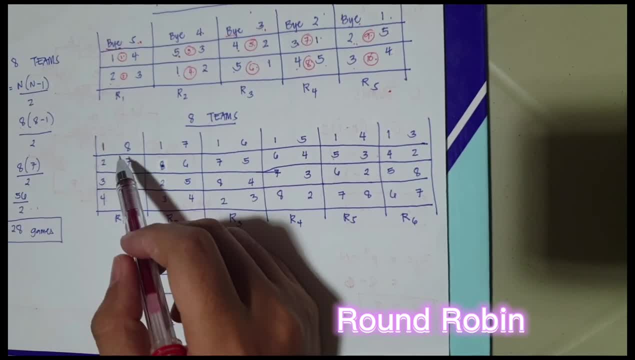 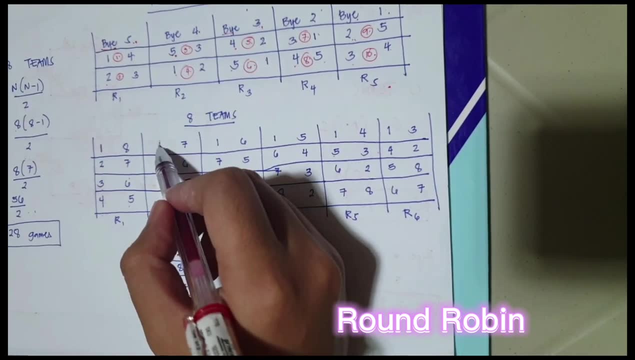 So meaning to say You're going to the direction to the left. Okay, So 1,, 2,, 3,, 4,, 5,, 6,, 7,, 8.. So 1, again 1.. So the next number is 8.. 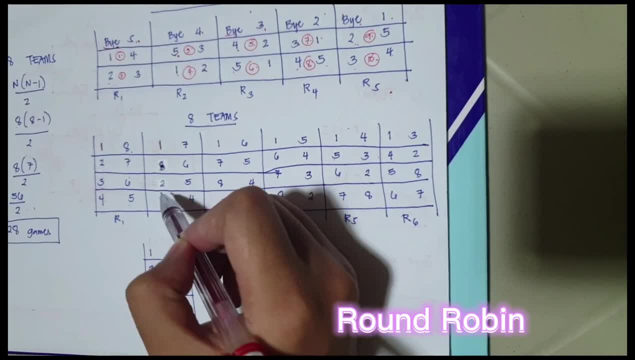 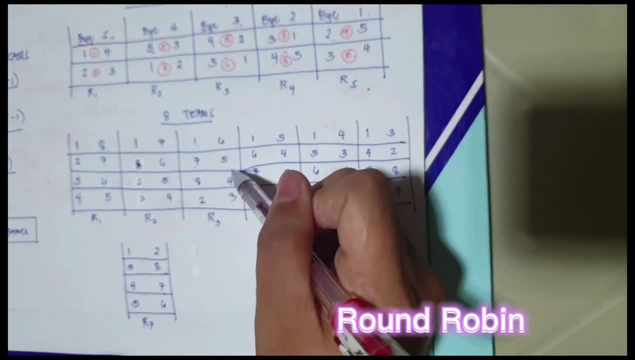 So the 8 is also below 1.. 2,, 3,, 4,, 5,, 6,, 7.. Then for the next round: 1, 7,, 8,, 2,, 3,, 4,, 5,, 6.. 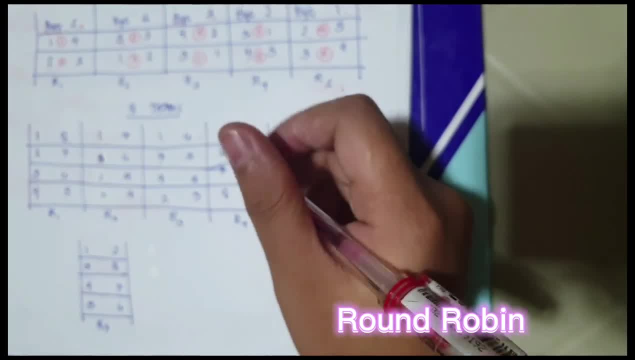 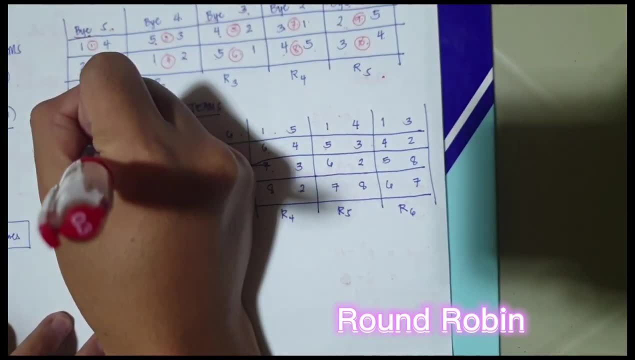 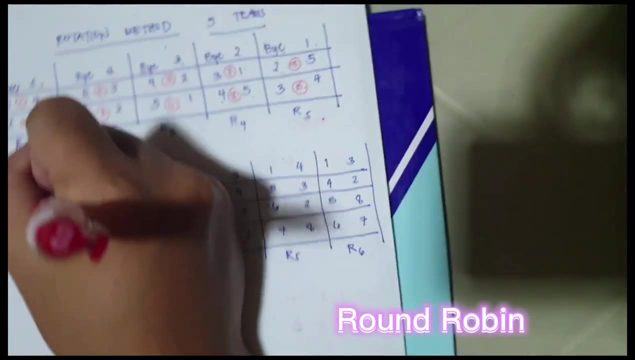 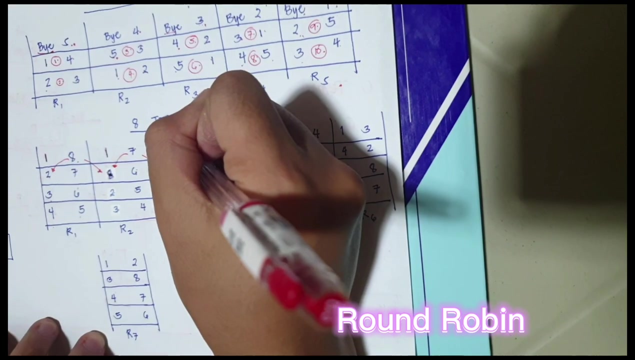 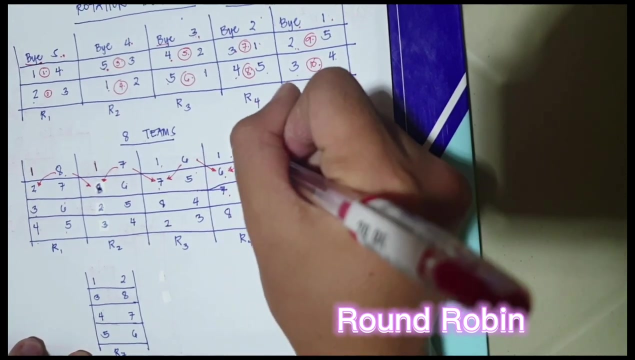 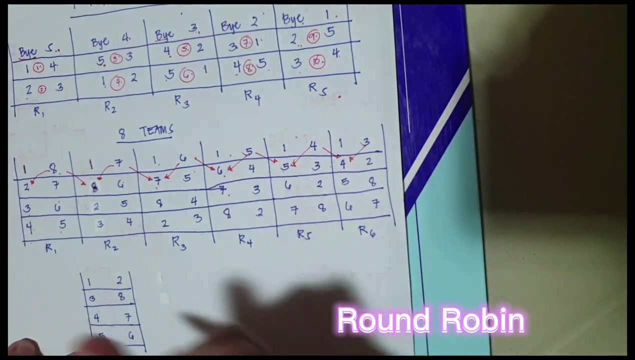 Then for the next round, 1, 6. 7, 8,, 2,, 3,, 4,, 5.. So, for example, 1, 8,, 2,, 3,, 4,, 5,, 6.. 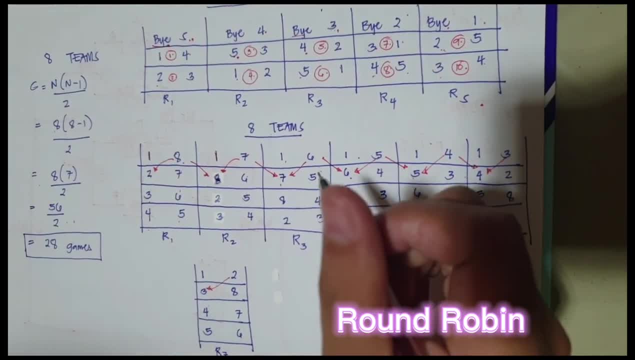 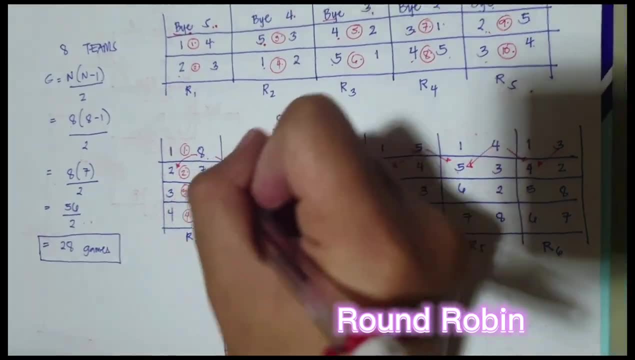 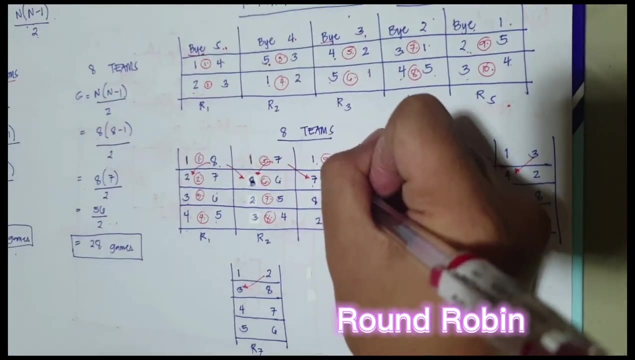 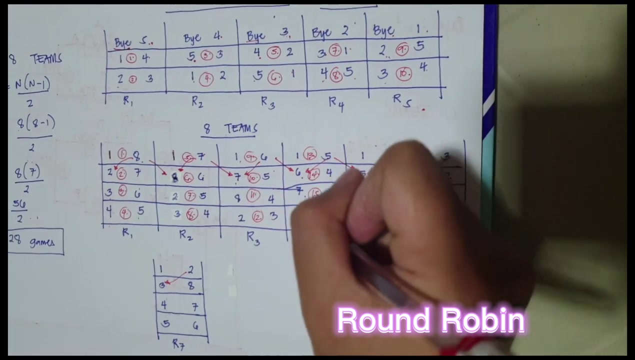 Okay, 1, 7,, 8,, 2,, 3,, 4,, 5, 6.. next is we're going to assign in a man the game number. so this is the game number one: two, three, four, five, six, seven, eight, nine, ten, eleven, twelve, thirteen, fourteen, fifteen, sixteen.